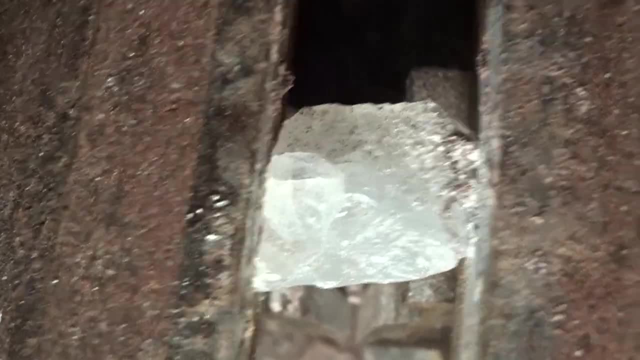 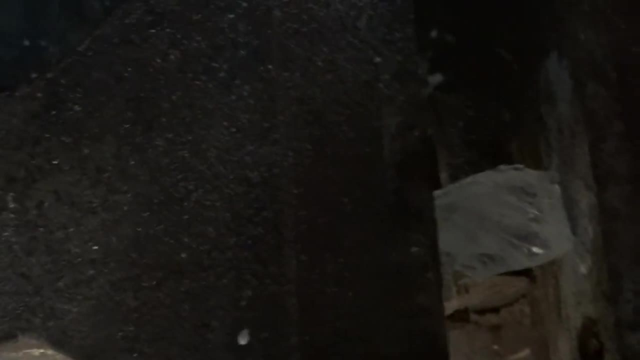 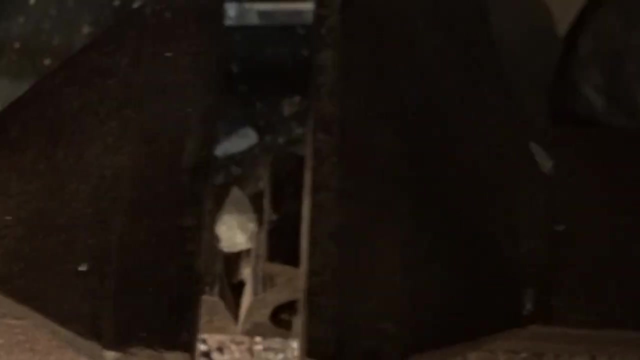 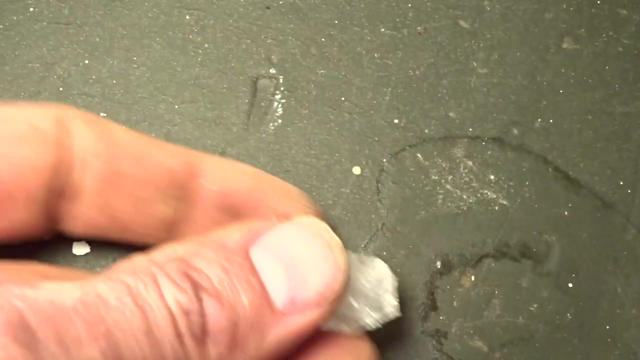 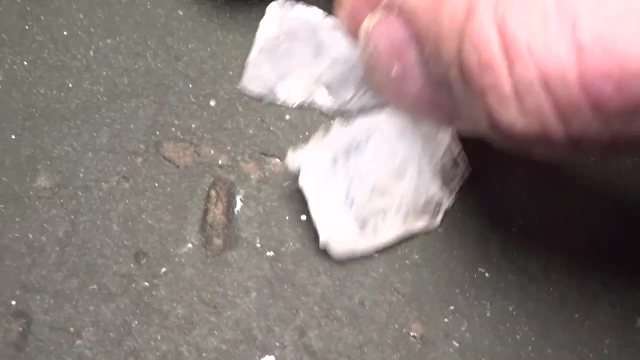 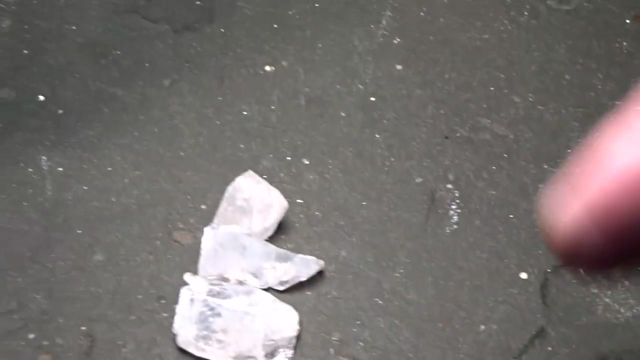 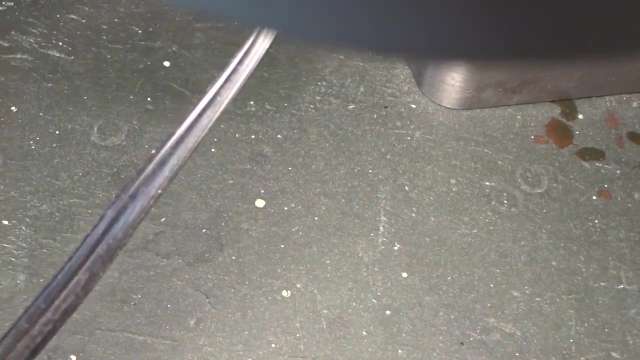 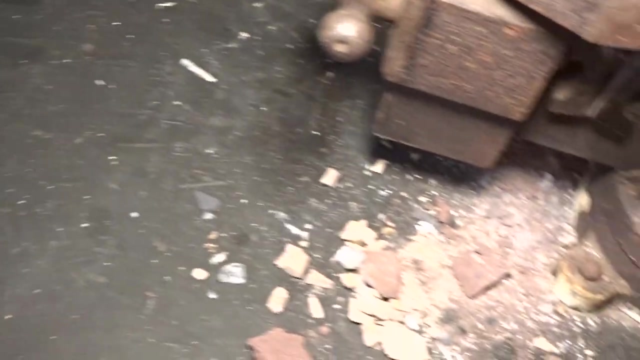 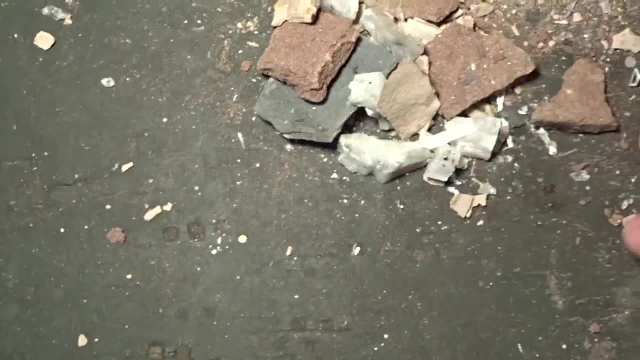 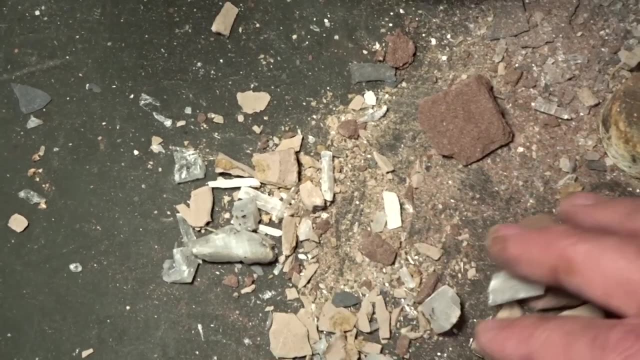 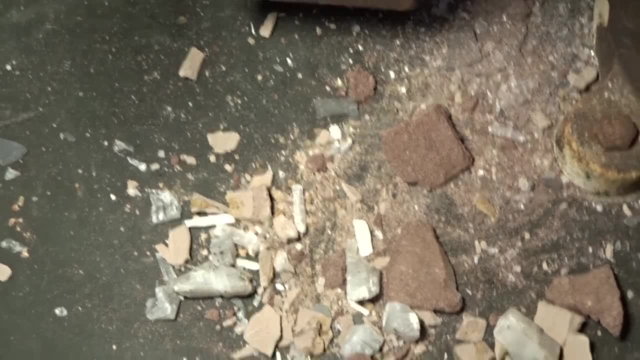 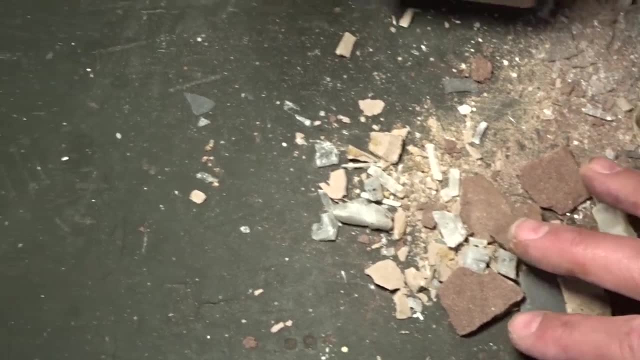 fracture and crack under pressure, under fracture and crack under pressure, under strain, under stress, under stress, when strain under stress, under stress, under strain, under stress, under stress, when they're strained under stresses strain. they're strained under stresses strain. they're strained under stresses strain under sustained load. 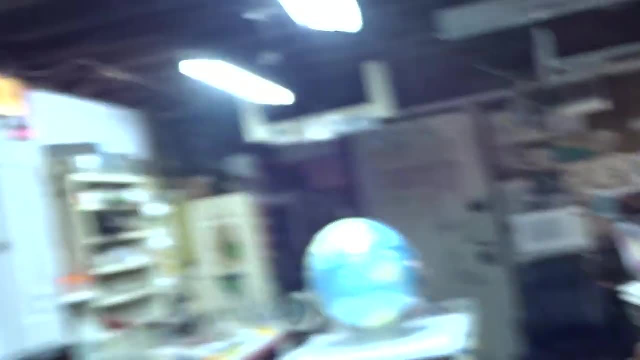 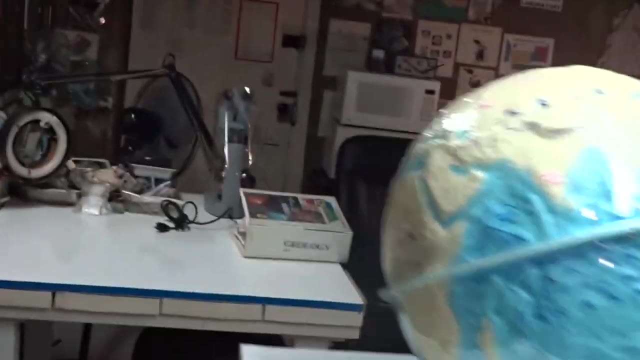 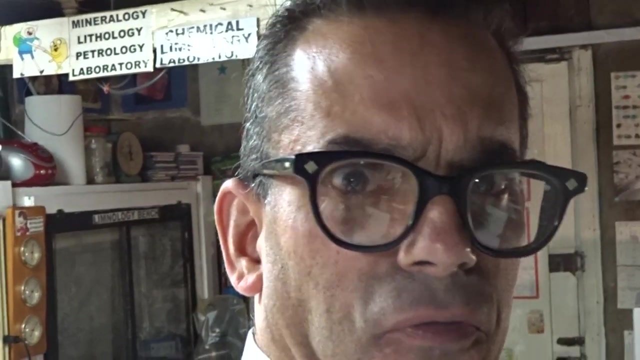 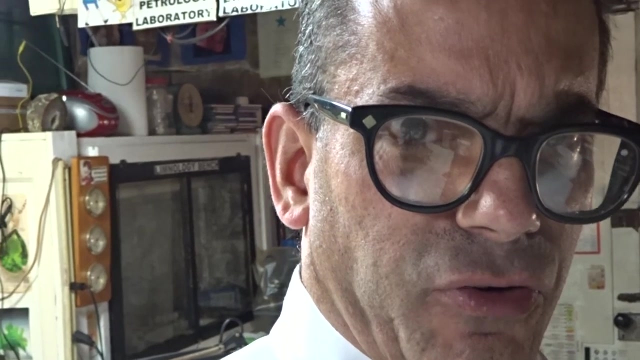